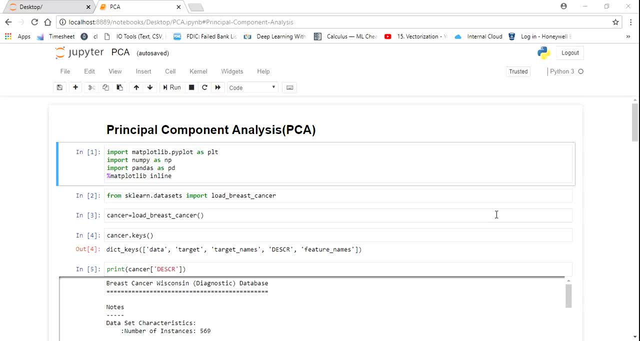 into two independent features by using a new vector space. at that time we can actually use this principal component analysis. so not only with three independent features, any number of independent features, and if you're trying to actually reduce those number of features to the number that you want, you can actually use this principal component analysis. so this technique. 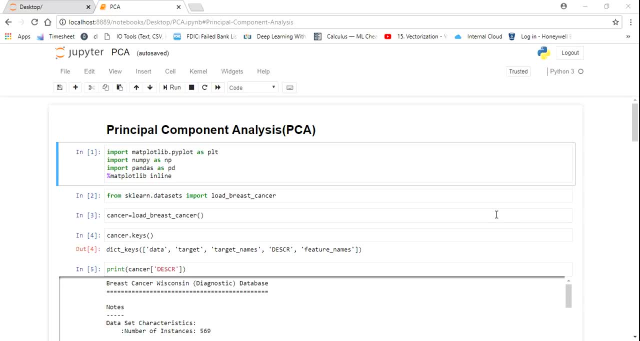 usually involves creating a lot of vector space, or you can say, no number of independent components. based on the components on or the number of dimensions that you want, we can convert any dimension into that particular dimensions. so before moving ahead, guys, please do subscribe the channel, because i don't want you all to miss any content. 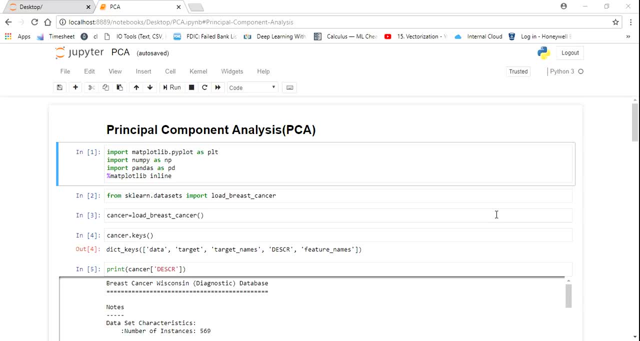 i try to upload as more as videos on saturdays and sundays, on every weekends, and i also upload videos on deep learning. so i'll try to upload one video on saturday on machine learning and on sunday i try to upload a video on deep learning. so please, before moving ahead, please do subscribe. 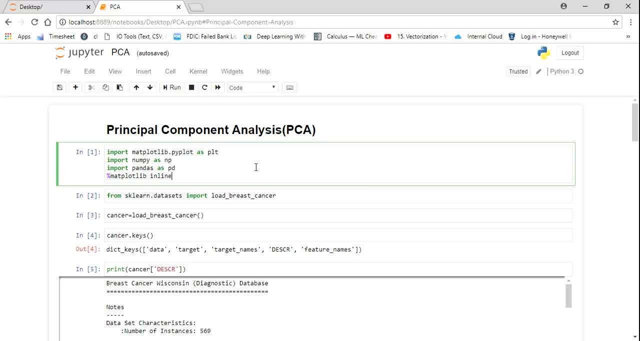 the channel. so now let me just move ahead with this principal component analysis. uh, so first of all i'm just going to import some of the libraries that i'm going to use, like matplotlib, which is used for actually plotting the diagrams, numpy, for creating arrays, pandas, to read the data. 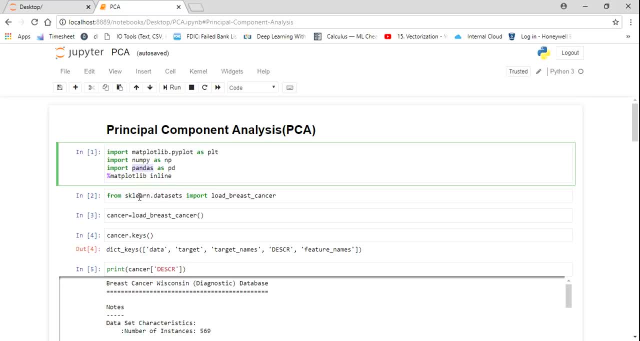 set. then uh, sklearn provides data set within itself from this library. i'm just going to import a particular library, a particular data set called as load breast cancer. so just let me execute this and show to you what this particular library is going to look like. data set has what is the details in this data set. so i'll just write load breast cancer with. 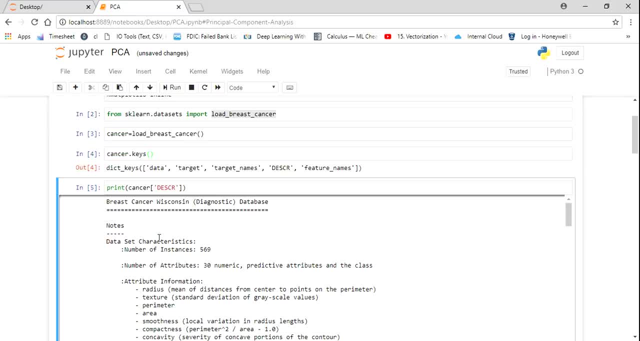 the method over here, and here is my cancer dot keys. when i execute the cancer dot keys, i have all these things. so i have all the data in this particular data key and my target is basically what is my output. so this is a basically a data set which says that what type of breast cancer it. 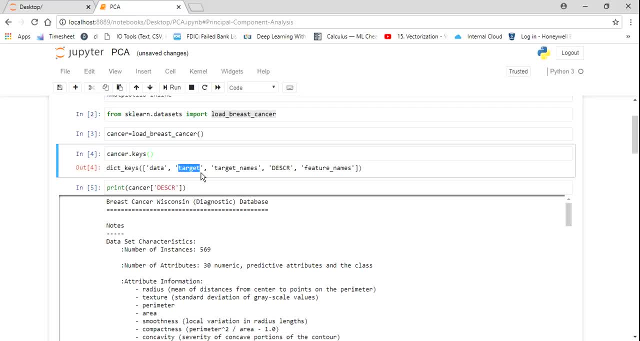 has. and if i see the target, there are two different types of target and we can see the description in this particular data set. here you can also pick the type of data set, for example. uh, i'm not going to duplicate names, okay, and there is also feature names. these feature names are nothing but. 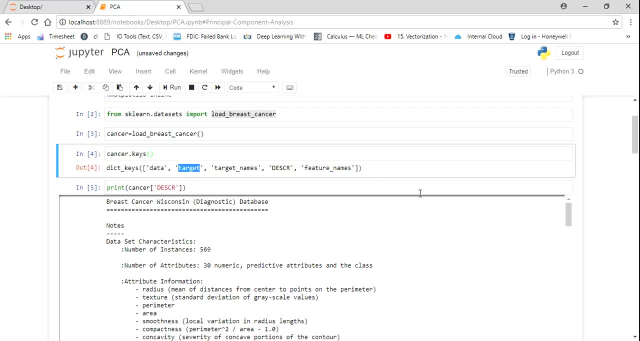 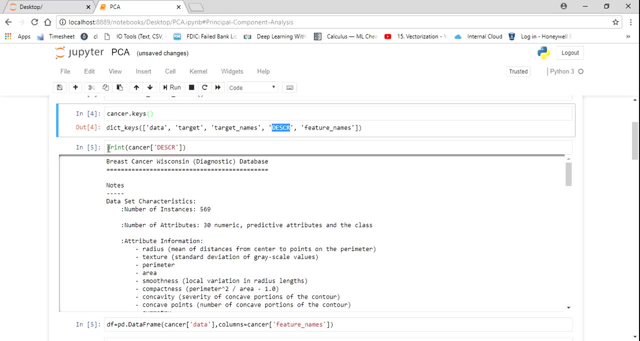 the data that we have, so all the columns. all the column name is having the feature names over here. okay, now you can also see the description of this particular data set from here, so you just have to write print: cancer, cancer of description. i'll be uploading this file in my github link, please. 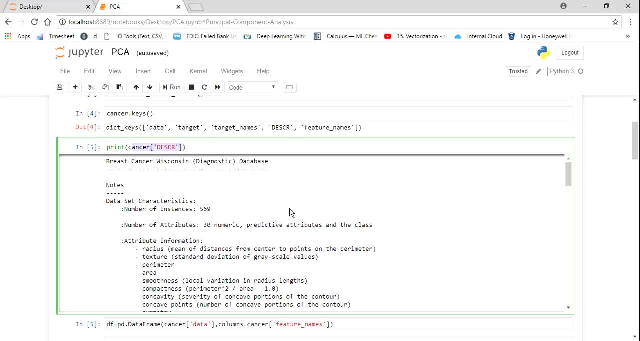 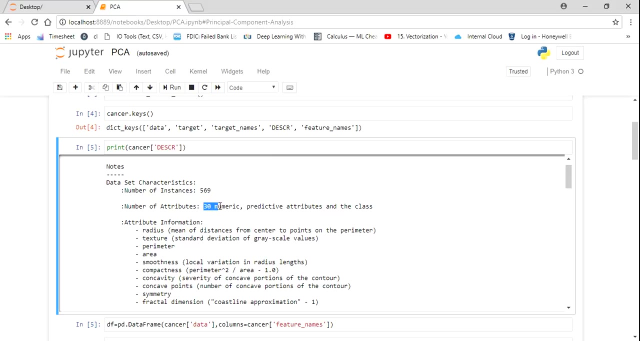 able to see the github link along with all this code. okay, so in this breast cancer diagnostic database you can see the description over here. so it shows basically like there are number of instances of so many records, how many different kind of attributes are there. this is basically. 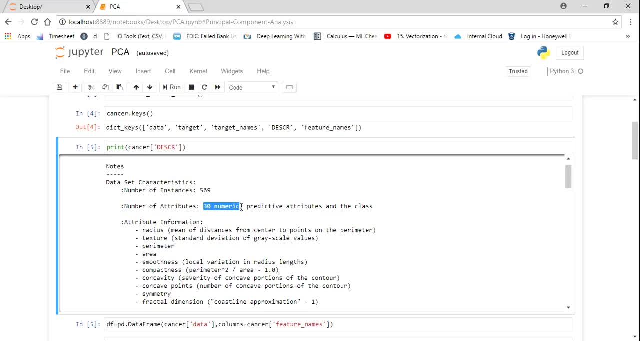 columns, right? so if i see a 30 numeric oem, that means 30 different independent features, so you can say this as a: it is 30 dimensional, okay, and we'll try to actually reduce this 30 dimensional into two dimensional and we'll see how well the new dimensions will be created by considering. 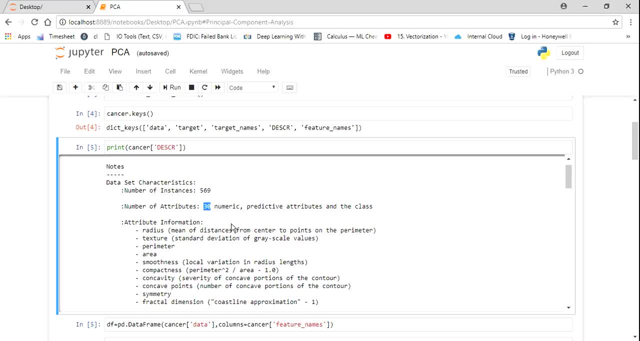 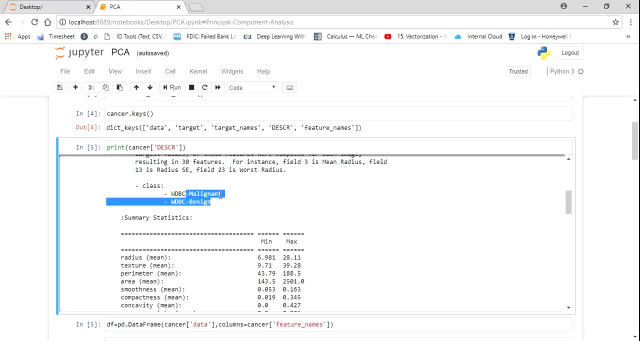 all these features, such that it will not lose that much amount of data also. okay, so you can see all these descriptions from here. and, as i said that there are two type of targets, names that one is malignant cancer, one is benign, so malignant, i think it is given a value as zero and one. so if 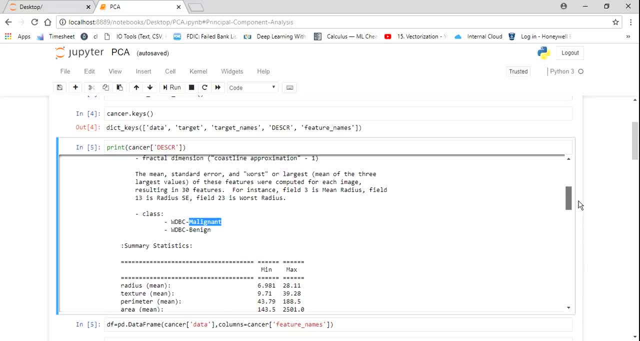 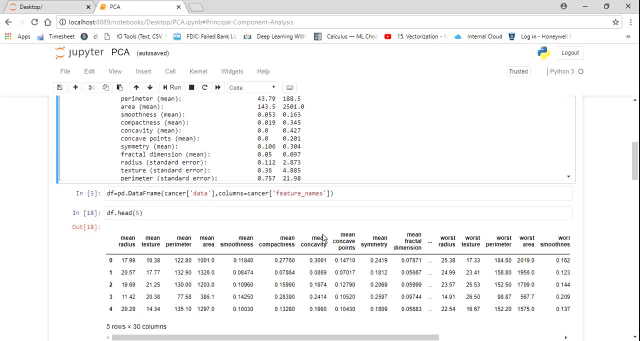 you see, if you just go down, there will be something called as target, i guess, or just let me display the target over here in the below. so what i'm going to do, i'm just going to create a data frame where i'll be taking pddataframe. my first attribute will be my data and the second attribute 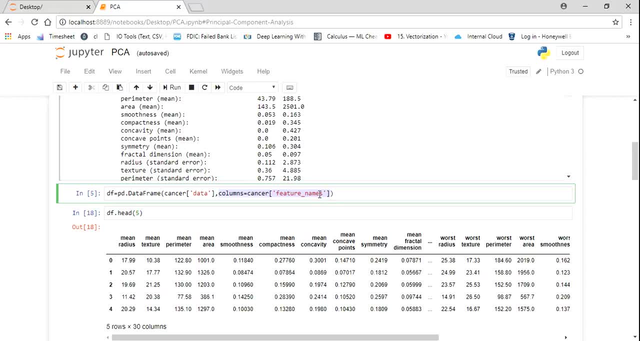 i'm going to put the column names, which will be my feature names, over here. okay, so all the feature names will be appended as my column names and it will be having all the data from this particular data key. okay, so once i execute this, i can see my data frame ahead as five. you can see all the features. 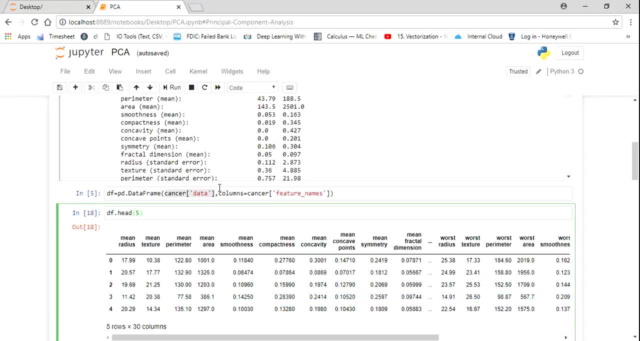 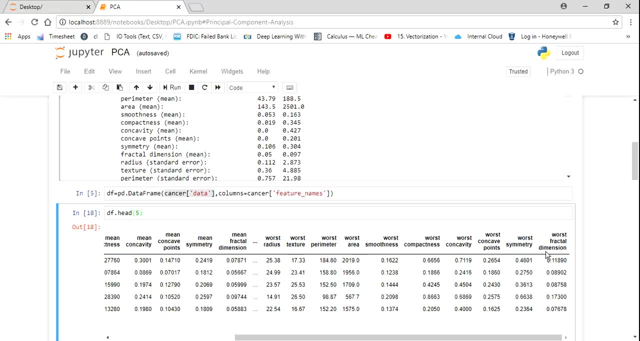 all the columns that have all the independent features over here and from this particular data value. we are getting all the values over here so you can see how many features are there. they're mostly around 30 features, as we saw from the help section, so these are the 30 features that we have. 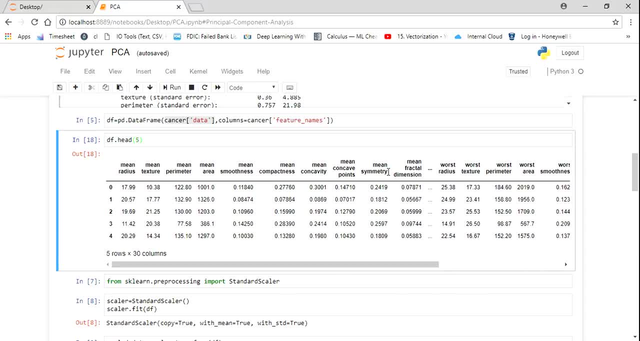 over here now. what we try to do is that, by using pca, we'll try to reduce this 30 dimensional into two dimensional, which will be creating a new vector space. okay, so always remember that in the pca, while running a pca, the first thing that you have to do is do the standard scaling, okay, the? 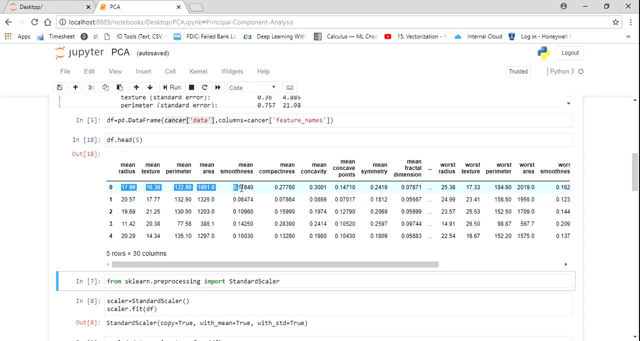 main reason is that you can see the values right. the difference between these values will be very high and if you are trying to create a new vector space, uh, the value should be. the difference on between this value should be very, very minimal. so for this purpose, i'm just going to use the 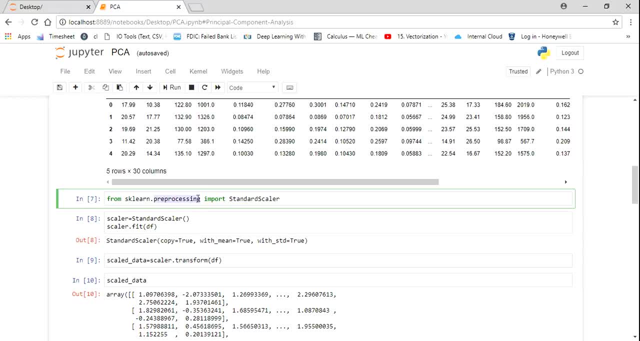 standard scalar. again, standard scalar is present in this sk learn dot pre-processing library. by using the standard scalar, as you know that by using standard, deviation is equal to 1 and mean is equal to 0, by that it will try to scale down all these values. you can also use min max scalar. 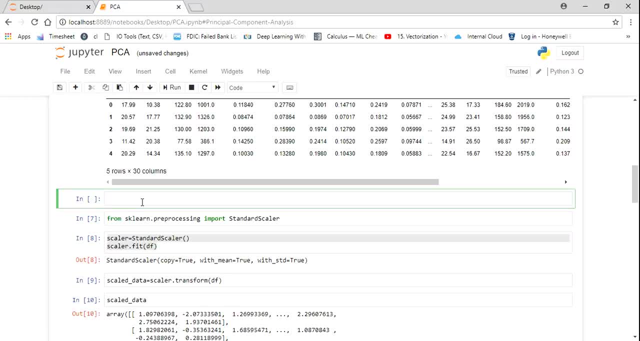 so suppose, if you want to use min max scalar, i'll just write it down for you so you can just write from sk. learn dot pre-processing. i'm just going to import min max scalar, so min max scalar will convert all your values between 0 to 1, right, so you can use. 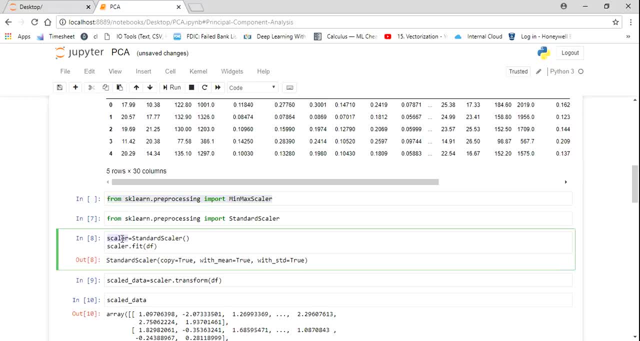 min, max scalar- and you can again do the same operation- initialize object and then do a fit operation on the data set. that's it, and with this you will be able to do the scaling again. i mean, to finish the scaling you need to also add and transform operation on the data set. 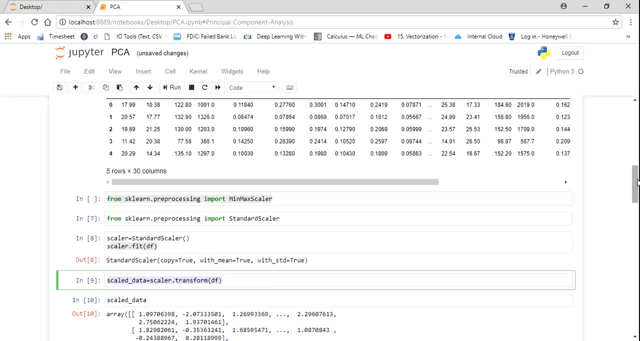 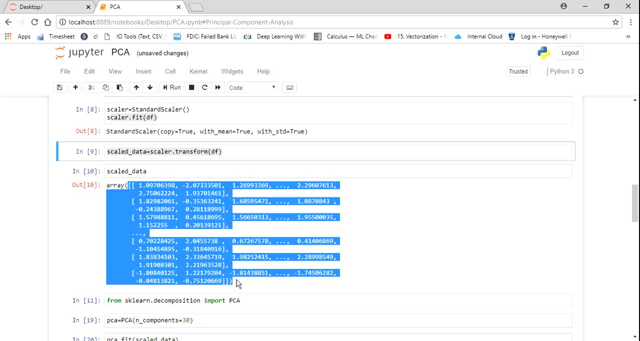 so once you do this, you will be able to do the scaling. okay, once i do the scaling, you can see that it has been converted into an array, and this is based on the standard deviation, as 1 and mean is equal to 0.. then, after this, you can up. 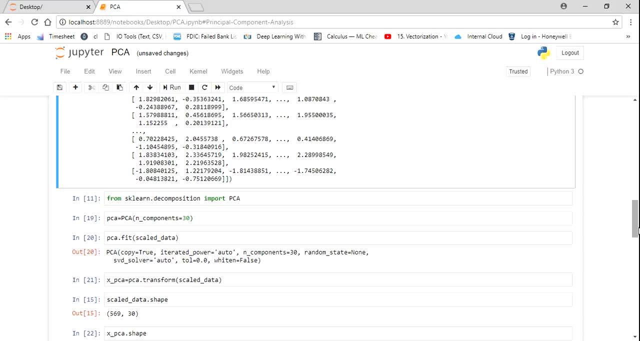 lie. now the pc algorithm. okay, sorry, the pca technique. uh, so, as i said, that pca technique, it is basically used for dimensionality reduction. so if i want to reduce the dimensions of 30 dimensions to 2, how can i do it? so i'll just write it as from sklearndecomposition. this is my 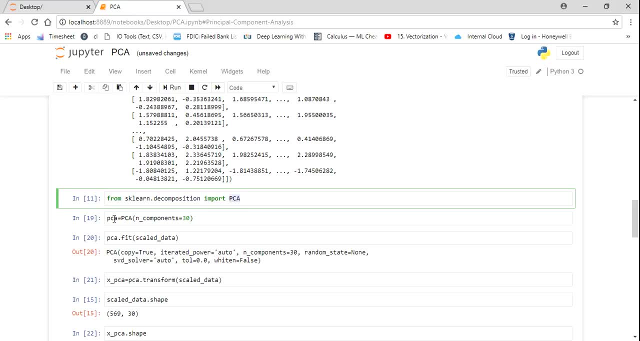 library. i'm trying to import this class called as pca. okay, in this pca, if i execute this pca and you can see that, if i press shift tab over here, you can see the. the first attribute is the number of components. this is the components. like the number of components you want to reduce. 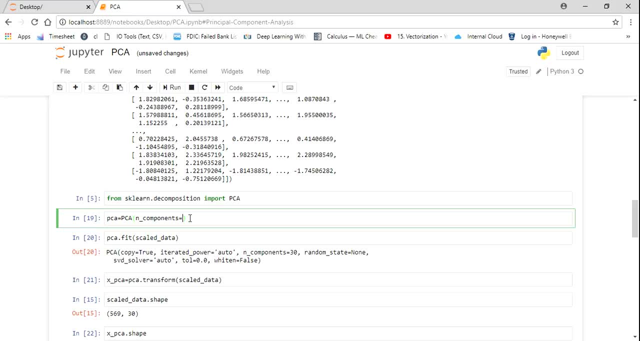 the dimension to. so from- uh, i mean from, from the total 30 dimensions. i want to convert this into two dimension only by using a new vector space. so my whole 30 dimensions, just understand my whole 30 dimensions getting converted into two dimensions. isn't it cool? yeah, so this is a wonderful features. 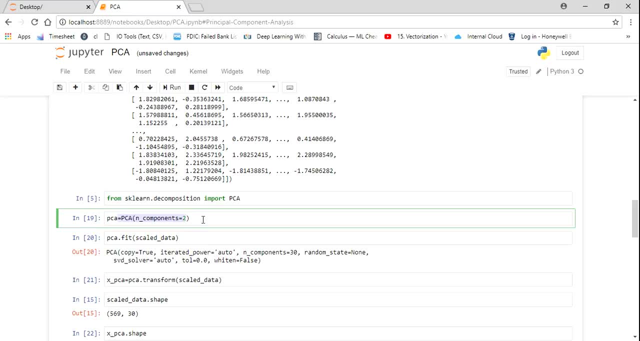 where you can actually convert so many dimensions. so if you have many dimensions right at that time, uh, usually uh provides an underfitting problem because because of those kind of dimensions the model will not be able to predict properly. so by this we are just using n components is equal to 2. 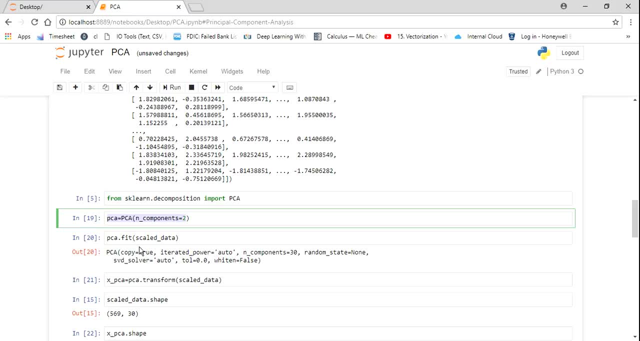 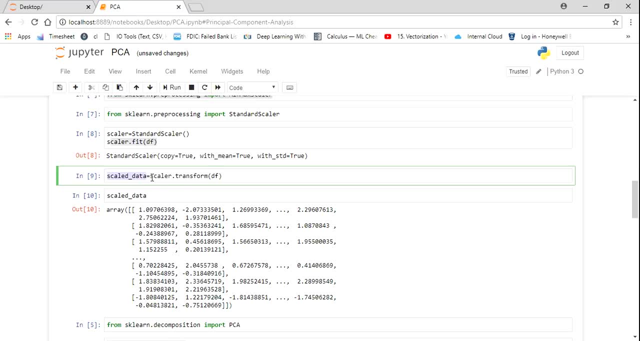 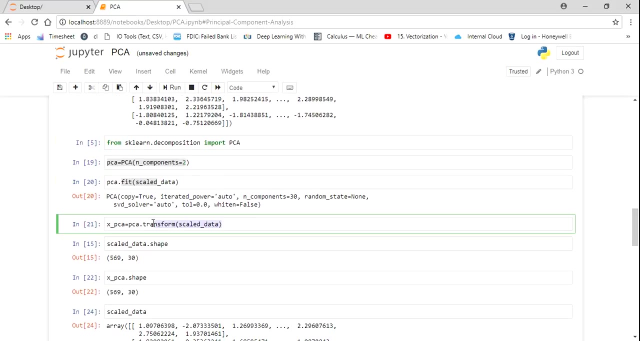 and i have created my pc object over here. okay, then i'm going to fit my scale data. the scale data is my this data, which i have scaled down by using a scale standard scalar method. okay, now, if i go over here i'm transforming the pca uh by using the pca object for the scale data. now you can see my scale data had a shape of 569,630. 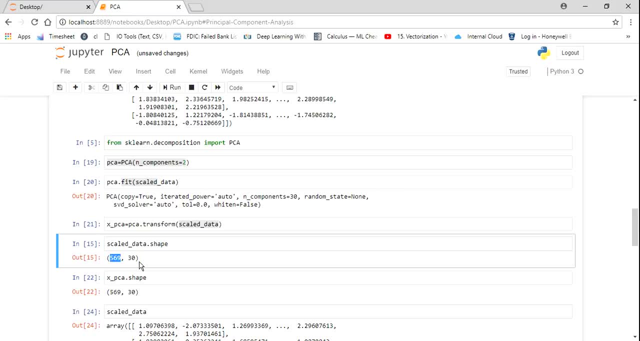 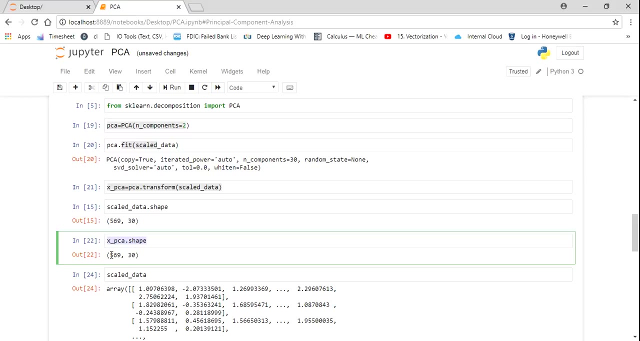 okay, 569 is basically my number of rows and 30 is the number of columns, so 30 was the number of different kind of features. now, after applying the pca technique, you can see over here for the variable x underscore: pca dot shape. when i did it it gave me around, so just let me execute this once. 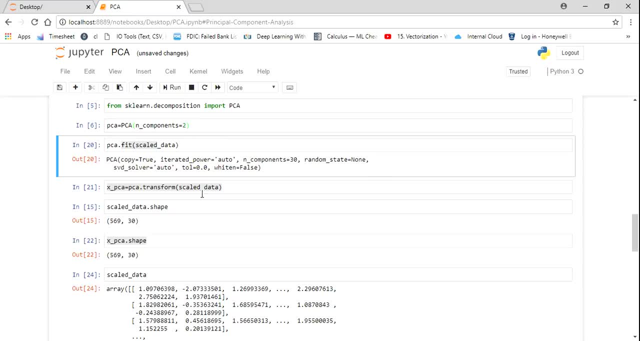 so, okay, just let me execute everything once again, because i was just trying to do something, so i'm just going to restart and run all so that it starts executing faster. just give me a moment, it will run off. okay now, perfect, now you can see that. oh yeah, i'm showing you the scale. data dot shape: right. 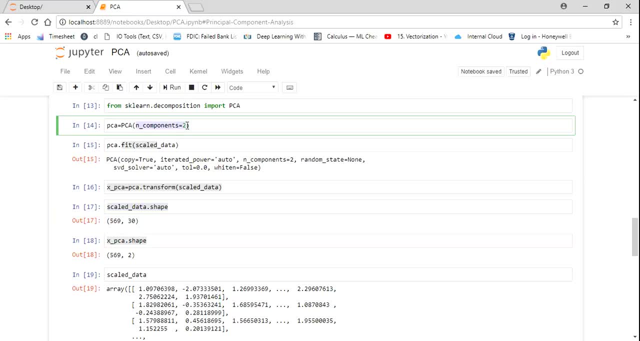 i have converted the dimensions into n. underscore component is equal to 2. okay, so that means my 30 dimensional is getting converted into two dimensions. now if i see my scale data dot shape, it is 569 comma 30.. that means i have 569 rows and 30 different dimensions, that is 30 independent. 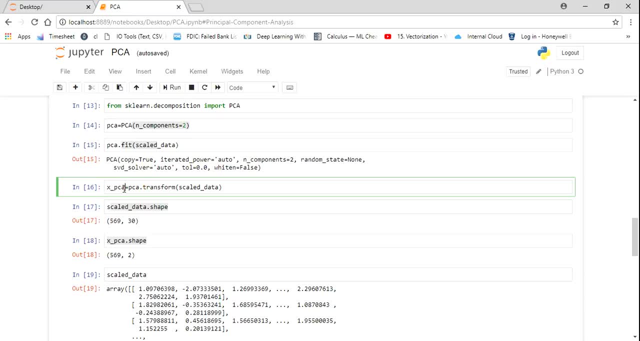 features. and now, after applying this transform method, i get this x underscore pca value. you can see the shape of this x underscore pca dot shape. it is 569 comma 2.. now see, say this: this 30 dimensions has got converted into two dimensions, so this is a very good way of reducing the 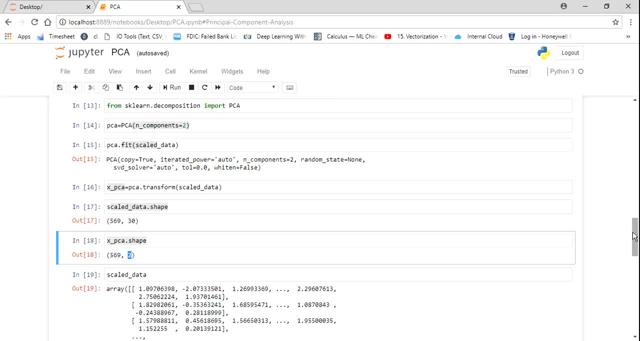 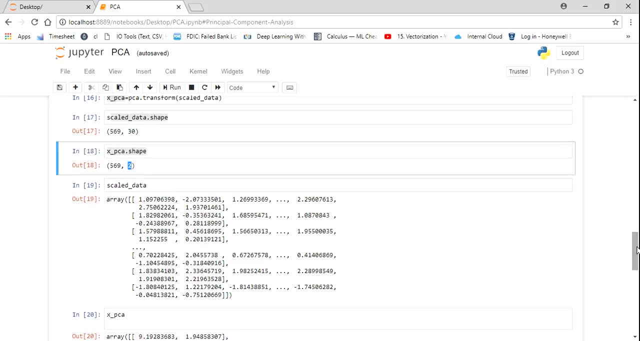 dimensions. once the dimension is getting reduced, you have the target value over there. you can apply any algorithm you want, like um. if you want, you can apply logistically linear regression or you can also apply some some kind of decision trees or any classification kind of algorithm to determine. 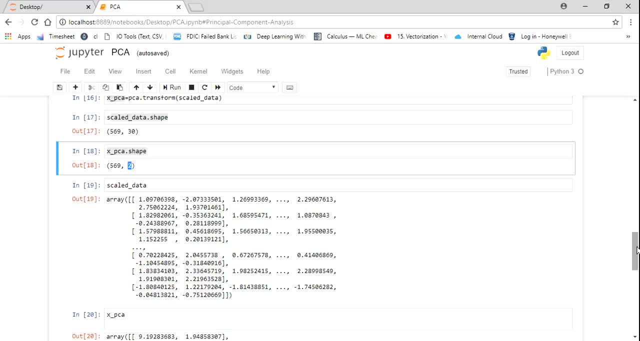 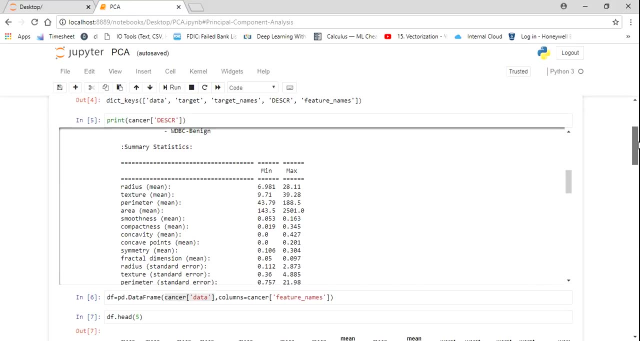 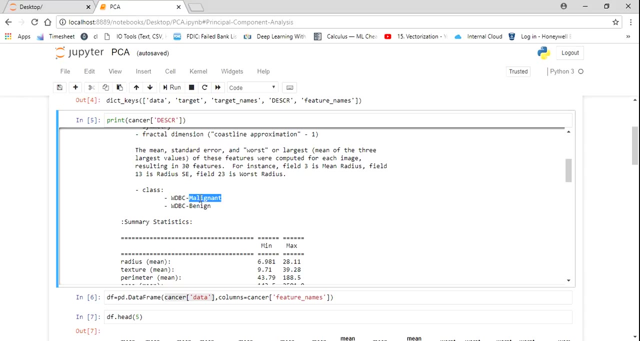 which particular uh target name it is of like, whether it is a, it is of mena or it is for. so if i show you my target names over here, whether it is my malignant or benign, okay, so based on this target values, you can then apply your 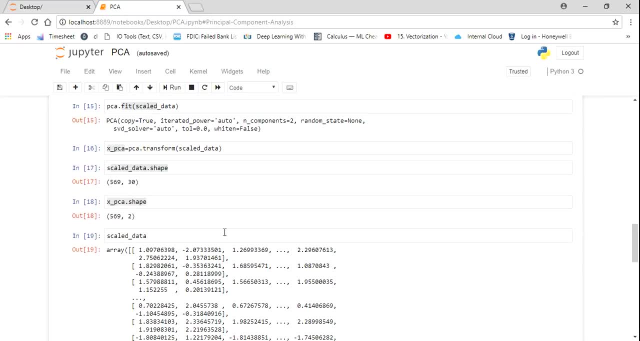 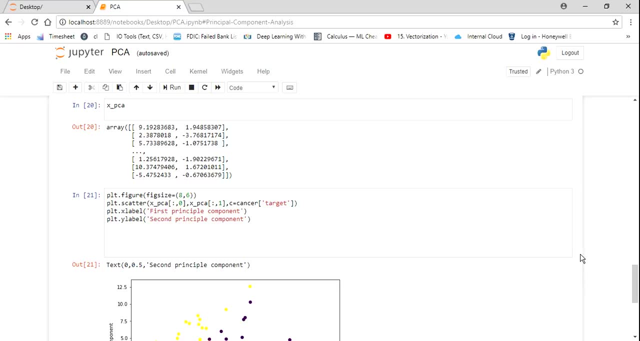 uh, algorithms for this x and x underscore pca dot shape. okay data. now let me just go down a little bit. you can see that i'm just creating a plot figure over here. i'm just plotting my x underscore pca. since i have two independent features, i'm going to plot it based on the target value, right? 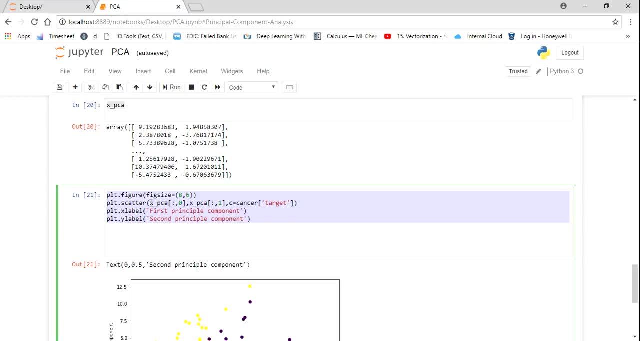 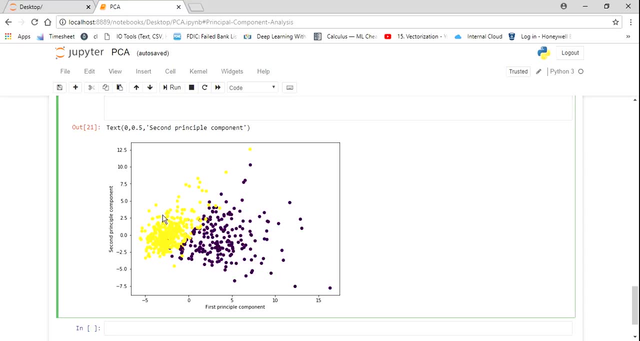 so, based on the target value, i'm going to plot this particular figure from these two particular dimensions. now you can see, even though the from 30 dimensions, this we have just created two dimensions. the splitting is perfect. you can see that. so it has not lost that much data. so it is. 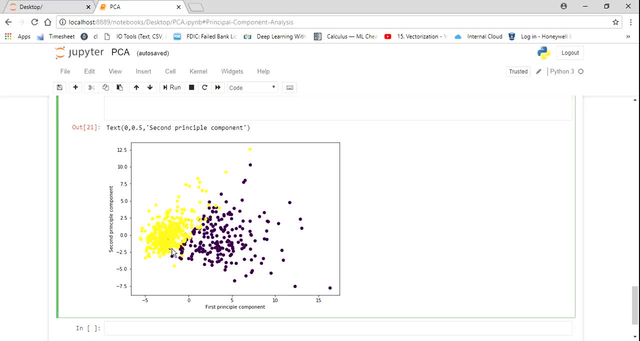 possible that you can actually don't worry about the number of dimensions that you have. okay, by using various, this principal component analysis, you can actually convert into any number of dimensions you want. now i have converted into two dimensions for a purpose because i could draw this diagram and show to you. so now this diagram: you can see that this is a zero values.